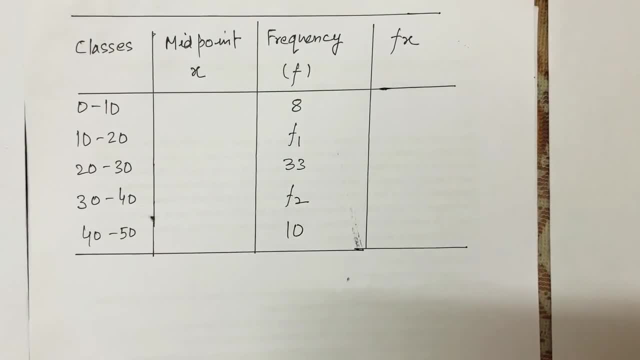 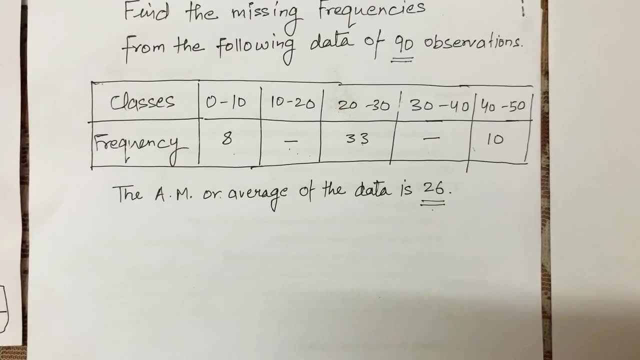 Hello everyone. so in this particular lecture I am going to discuss a problem which is of missing frequencies. So here is the problem right in front of me. if you could see the problem right here. The problem is about I have to find the missing frequencies from. 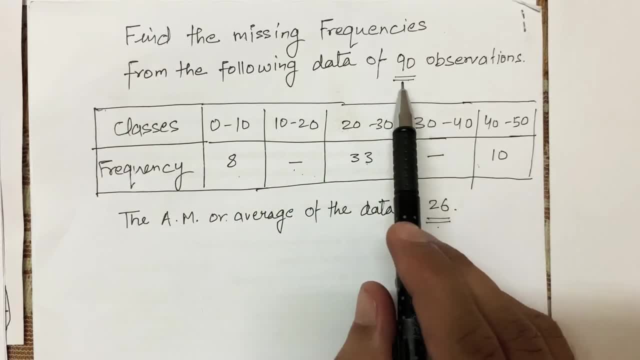 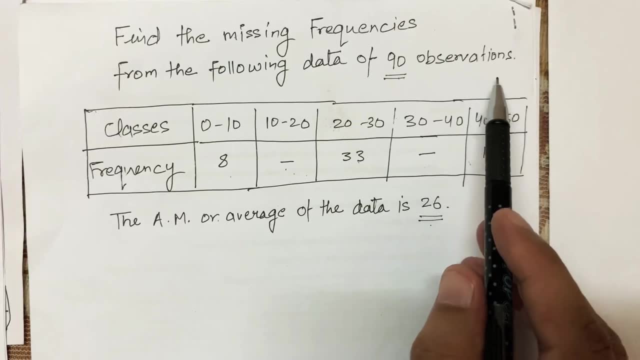 the following data of 90 observations. So I have underlined the 90 observations. this is one of the important inputs which I will be using. So there are in total 90 observations are there and also the arithmetic mean of the data is given 26 and if you see the data, 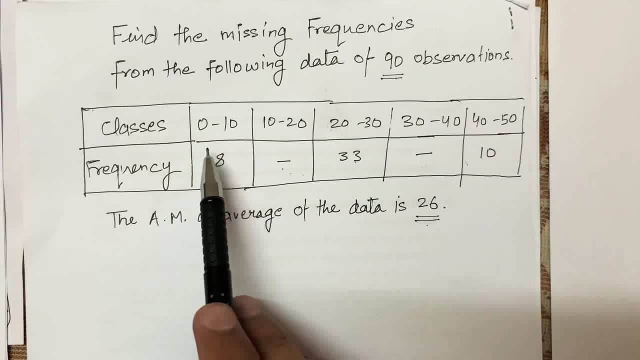 there are 2 frequencies which are missing. I know that how many students are falling, or how much data is between 0 to 10, 8,, 10 to 20. I have not been given with the data. 20 to 30- no data. 30 to 40- no data. and 40 to 50 is 10,, 20 to 30, there is 33.. So I need. 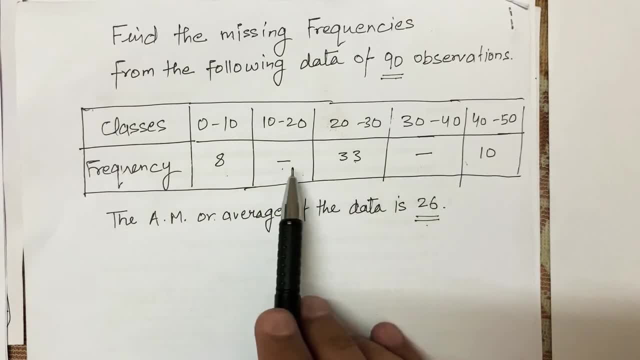 to find out what are these missing values? So, once again, let's focus on the input. if I want to find out 2 missing frequencies, I must have shown the data which is given, have the total number of observation and i must also have the arithmetic mean. let's solve this. 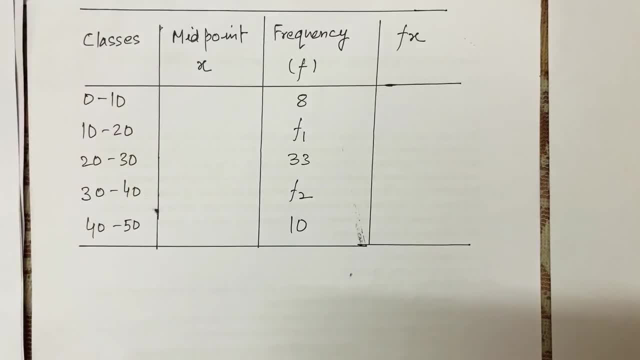 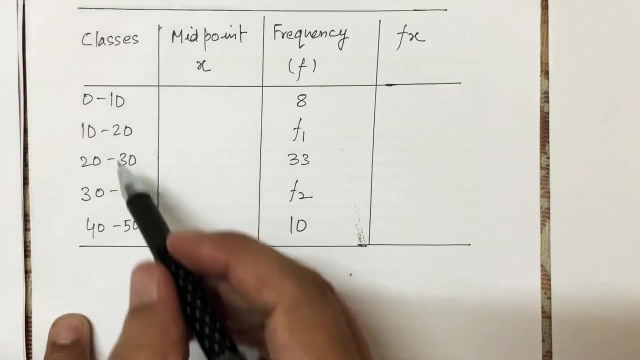 problem. it's a little complicated arithmetic mean problem. so if you see this whole structure, i have just put up the whole question, which is given in a tabular format, in a solvable tabular format rather, and so i have been given with the classes, i have been given with the frequencies. now, if you could, 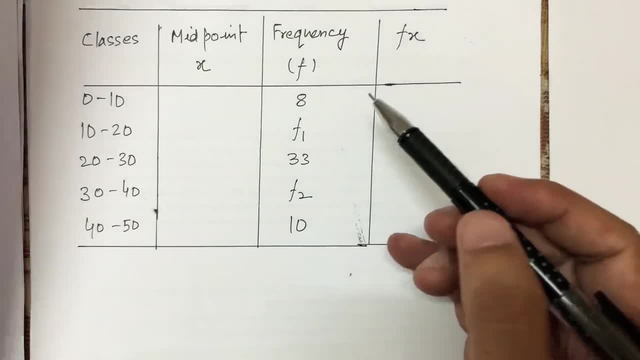 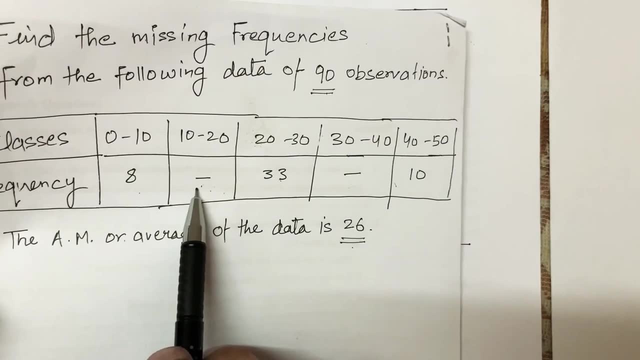 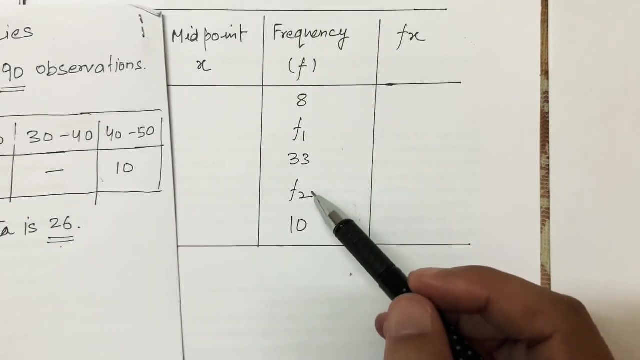 see, i have given, you know, two different symbols i have allotted to missing frequencies. so if you see it here that 10 to 20, there was no frequency, so i have given it a symbol f1 to add 30 to 40, there was no, there is no frequency, so i have given it a symbol f2 and that's all the frequencies. like 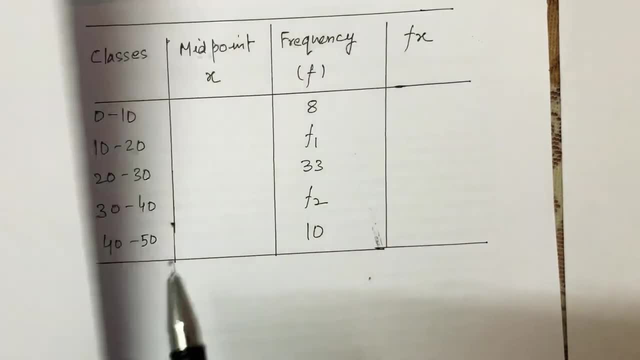 8, 33 and 10. they remain same: 8, 33 and 10. let's solve this particular problem. i will also write the important inputs here. okay, let me let you see the important inputs here. okay, let me let you see the important inputs here. okay, let me. 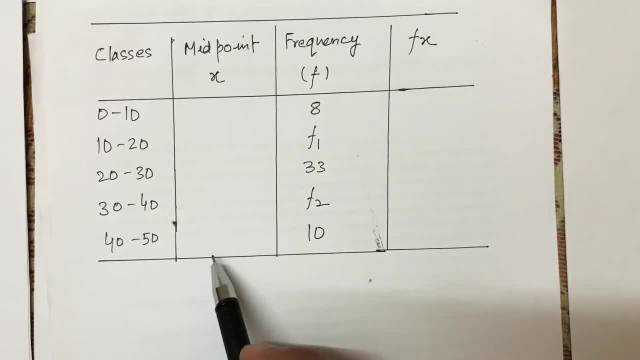 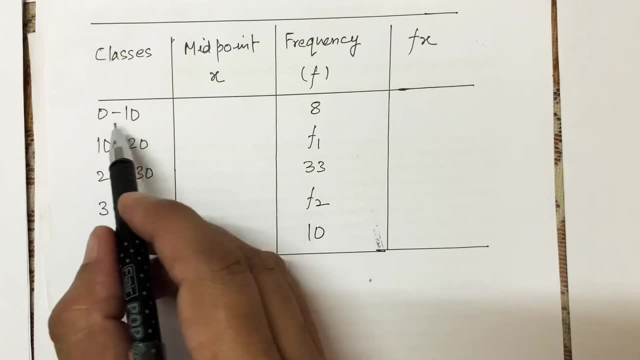 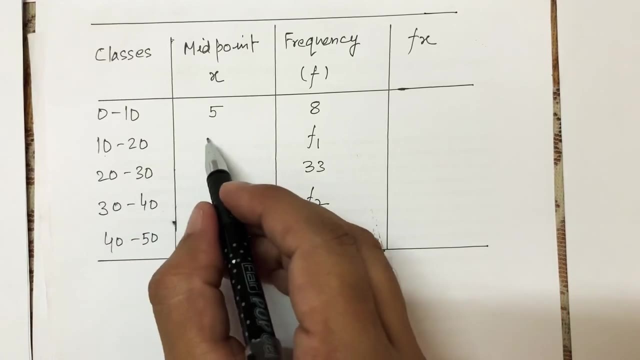 write them later. so first thing is i need to find out the midpoints in order to calculate the arithmetic mean. so the midpoint is upper limit of the class plus lower limit divided by 2, as discussed earlier. so 0 plus 10 divided by 2, which is 5 in this case. in this case, it is 20 plus 10 divided by. 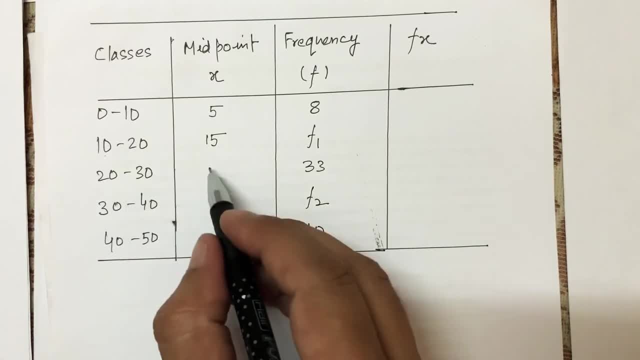 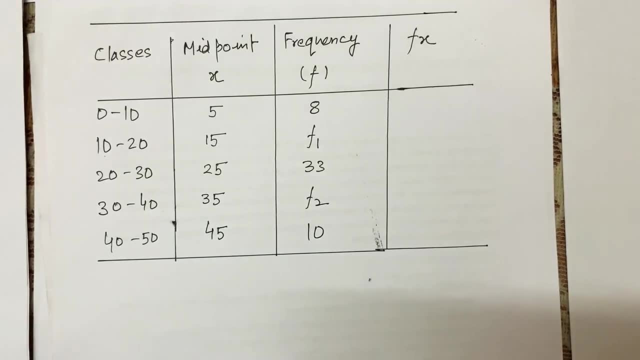 2: 30 divided by 2 is 15.. 30 plus 20 divided by 2 becomes 25, this becomes 35 and this becomes 45. so i have calculated all the midpoints right here. I will keep the process exactly same as we do in the arithmetic mean. 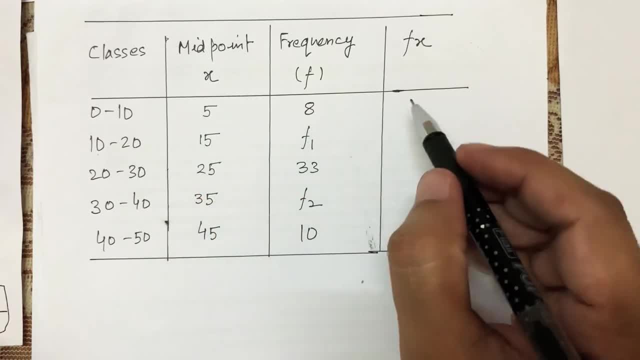 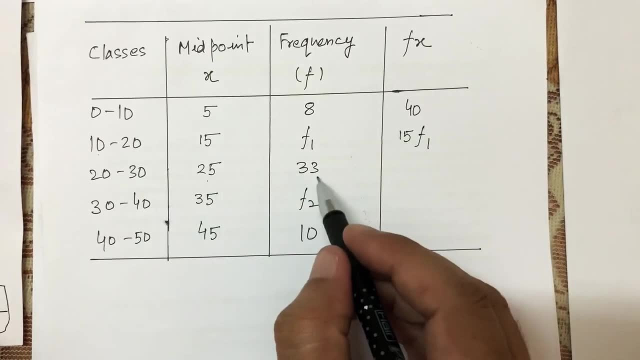 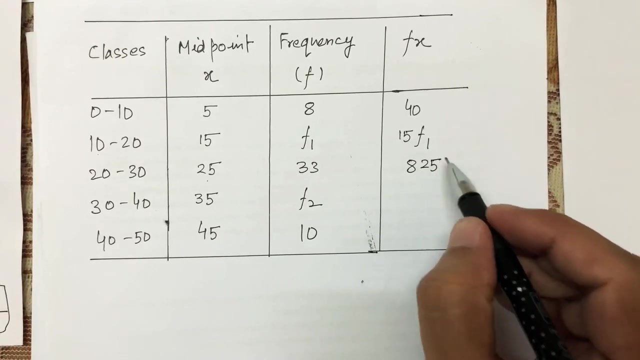 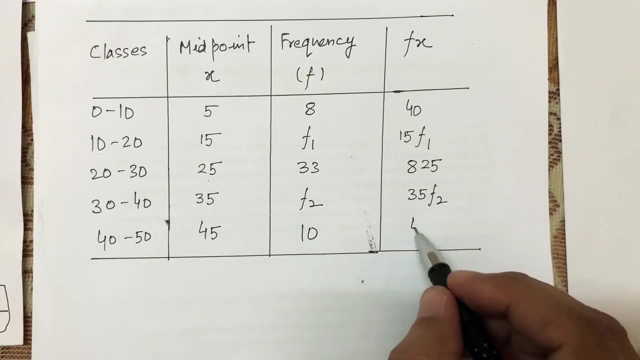 I have to calculate fx here: 8 times 5 is 40, This value becomes 15 of f1, 25 times 33 becomes 825, And here it becomes 35 of f2, and 45 times 10 becomes 450. So I have calculated fx throughout. Now, as you could recall, in the arithmetic, 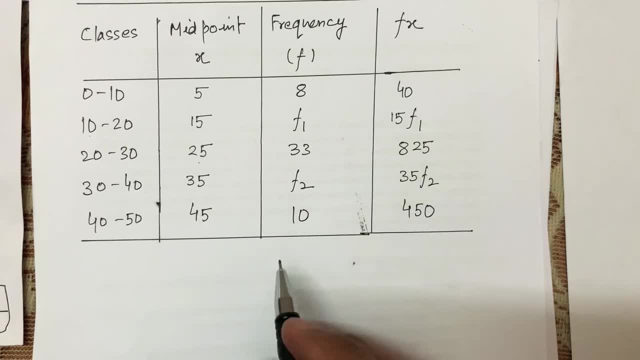 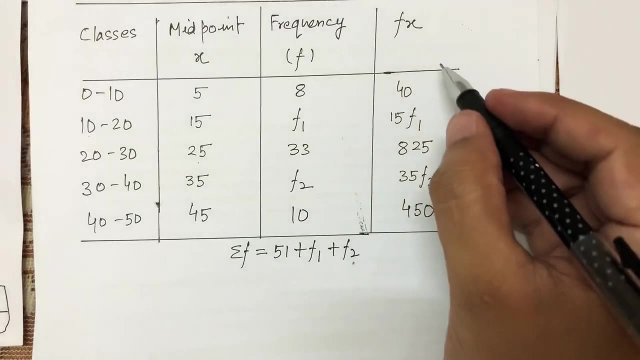 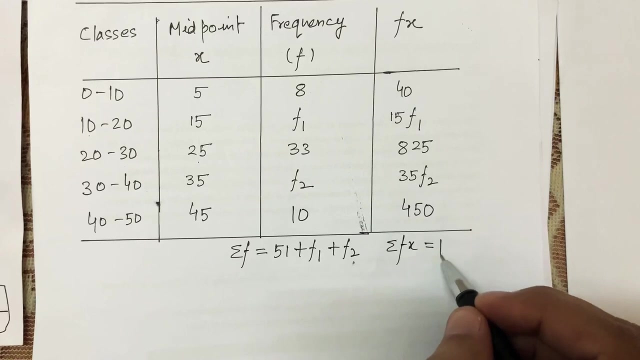 mean formula. I need summation of fx and summation of f. So what is going to be summation of f here? That is going to be 8 plus 33 plus 10, which is 51 plus f1 plus f2. And what is summation of fx? here It is 450 plus 8, 25 plus 40, which is 1315. 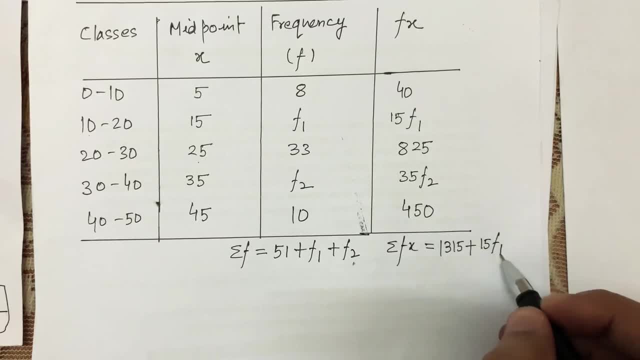 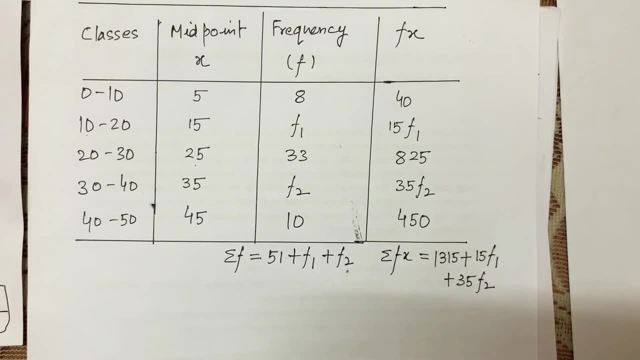 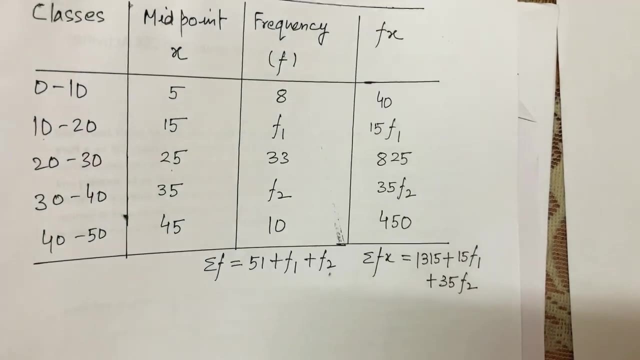 plus 15 of f1, plus 35 of f2. So these two important summations, which is to be used in arithmetic, mean formula I have. So I am going to use these two particular values to calculate the missing frequencies. I will just shift the sheet a bit up And I will keep the values. 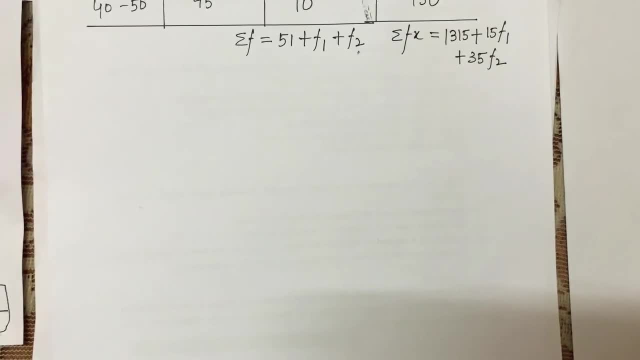 with me. So I am going to use these two particular values to calculate the missing frequencies. I will just shift the sheet a bit up Which I am going to use in tact. So there will be two equations which will be producing with the important values. The first thing is how many total observations? 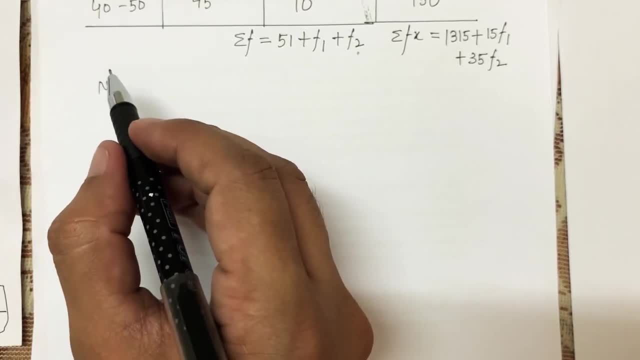 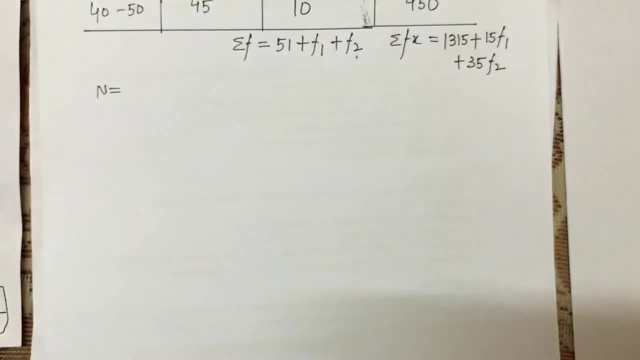 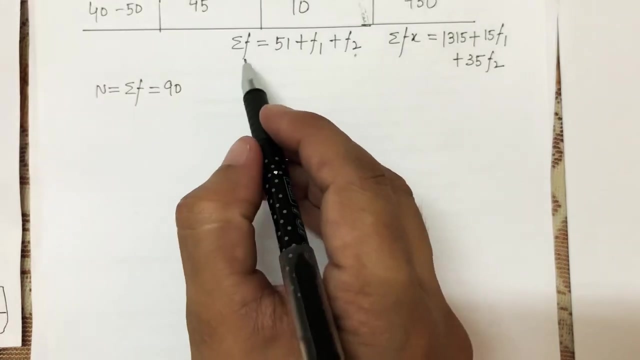 I have. It has been given in the question that total number of observations are 90. So I will just show: in the question it has been given that total number of observations are 90, So I am going to keep n or I can also write it. Summation f is 90. Now you look at the first particular input. 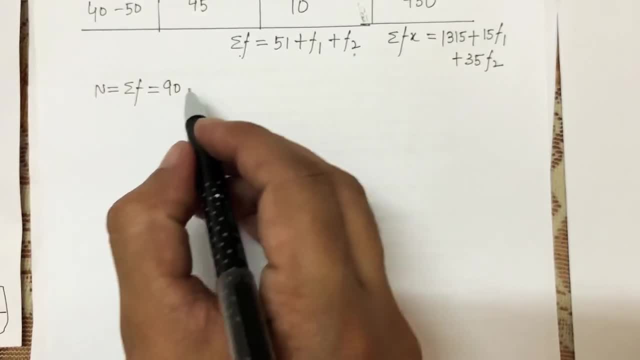 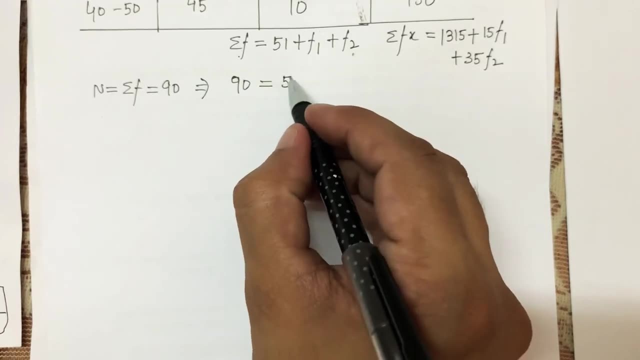 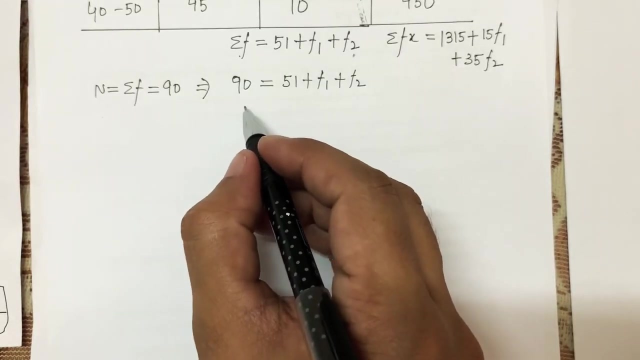 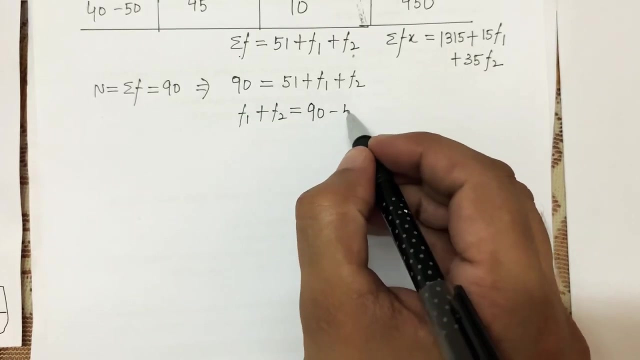 right here. What is summation f 90? So what it will become. So look at this. This implies summation of f is equal to 51 plus f1 plus f2. So from here what do I get? I get f1 plus f2, 51. I will take on other side 90 minus 51 And my first equation becomes: f1 plus f2 is. 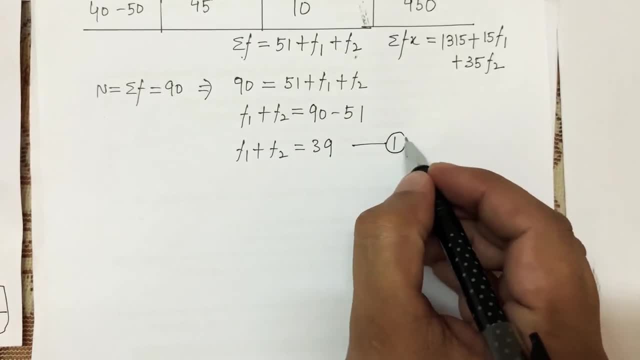 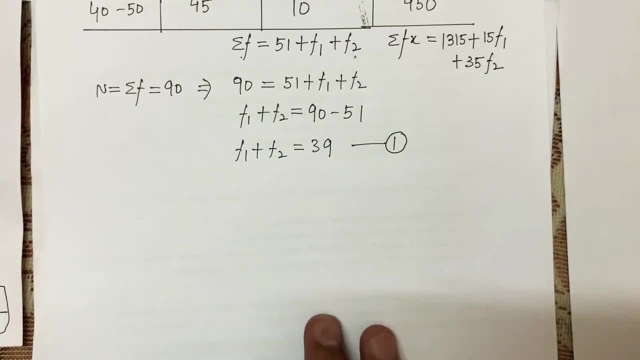 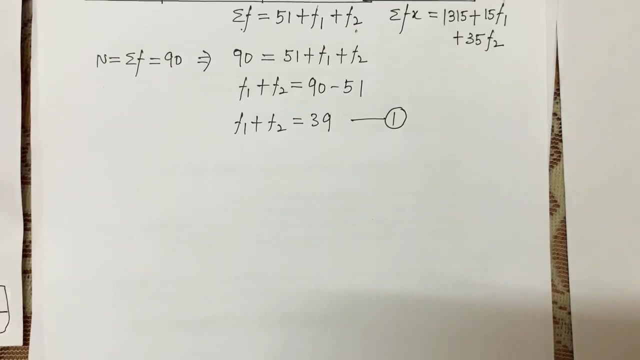 equal to 39. This is my equation number 1. So this is first important calculation in order to calculate two missing frequencies. How to get the first equation? You just use the concept of total number of frequencies And that is it: you get the first equation. Now let us see the other equation. 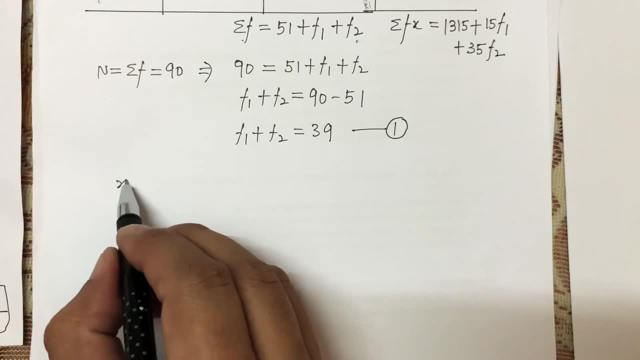 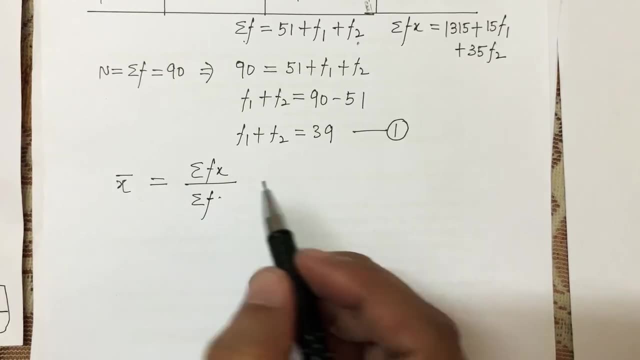 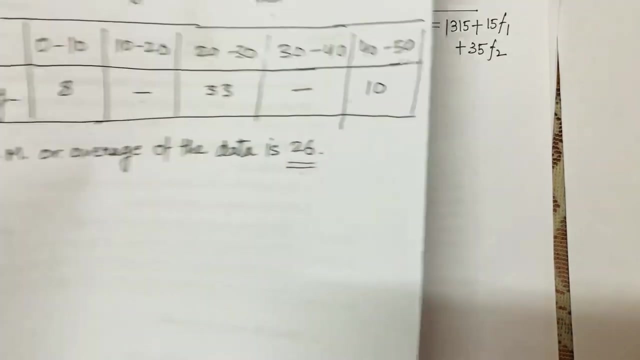 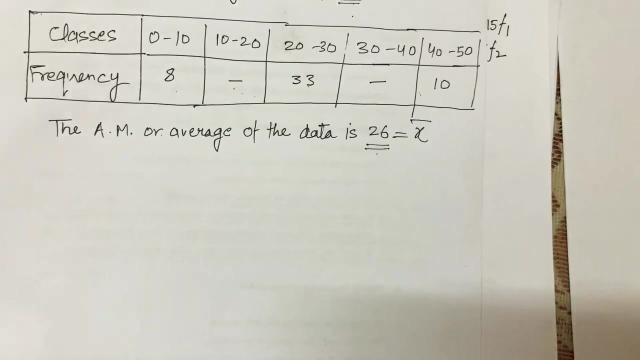 So I know the formula for x bar. It is summation of fx divided by summation of f. Now, if you look into the whole detail I have again been given in the question that summation of x bar, that means the arithmetic mean, is 26 And this is the value of x bar actually. 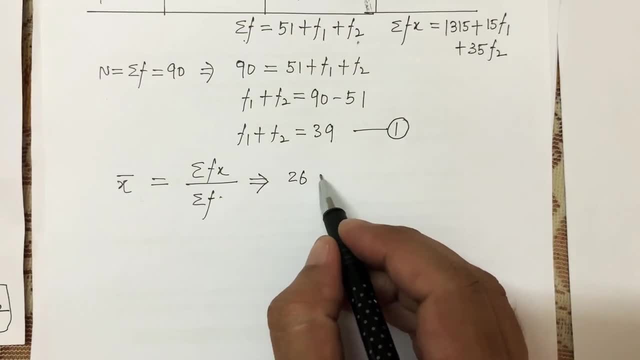 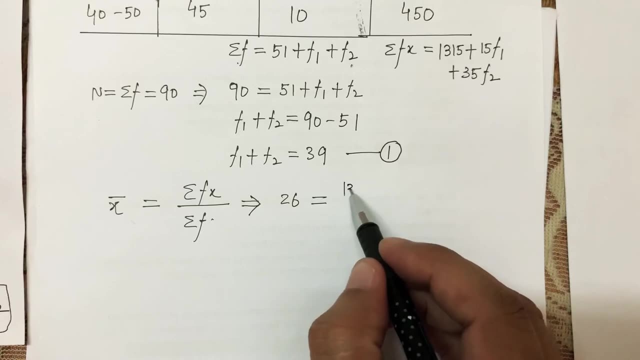 So I am going to replace x bar here by 26- is equal to: Now: what is summation of fx? It is right. here You could see that It is 1315 plus 15 of f1 plus 35 of f2, divided by f1 plus 15 of f2. 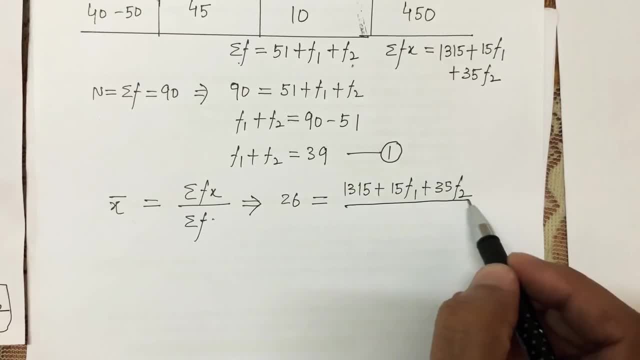 So I have again been given in the question That summation of x bar, that means the arithmetic mean is 26 And this is the value of x bar actually is equal to sum of f. x bar times x bar divided by sum of f, What is sum of f 90? I will do a little cross multiplication here. 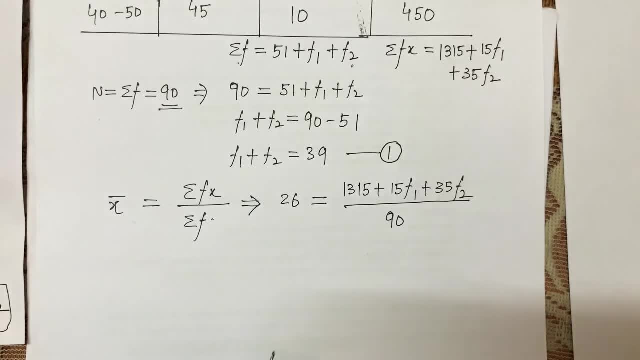 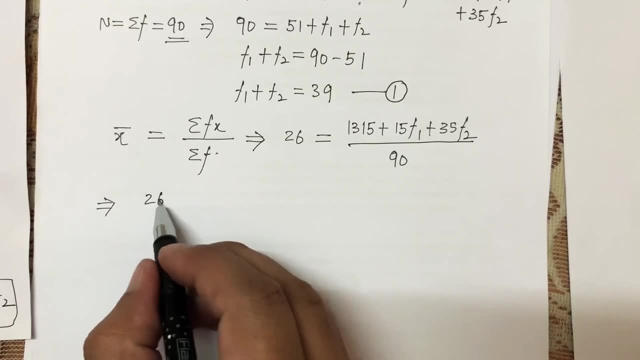 now That means that 90 I am going to take on left hand side. that is going to become 26 times 90. I will shift the sheet a bit up, So it is going to be now how it is going to land up. 26 times 90 is equal to 1315 plus 15f1 plus 35f2. 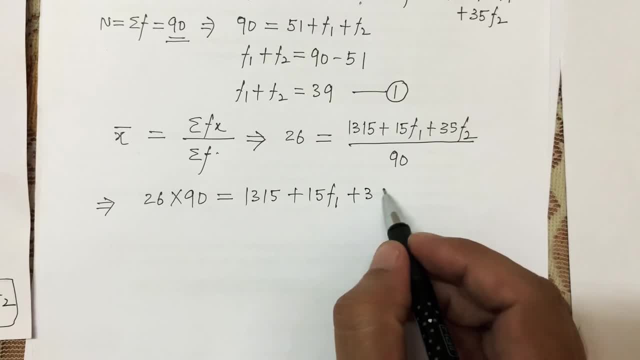 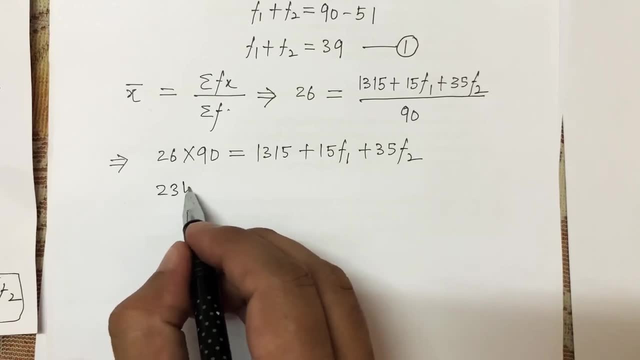 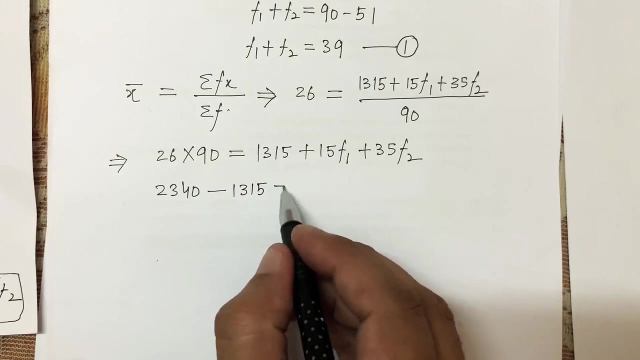 plus 15 f1 plus 35 of f2. now what is 26 into 90? it is 2, 3, 4, 0. I also take 1315 on the left hand side. minus 1315 is equal to 15 f1 plus 35 of f2. 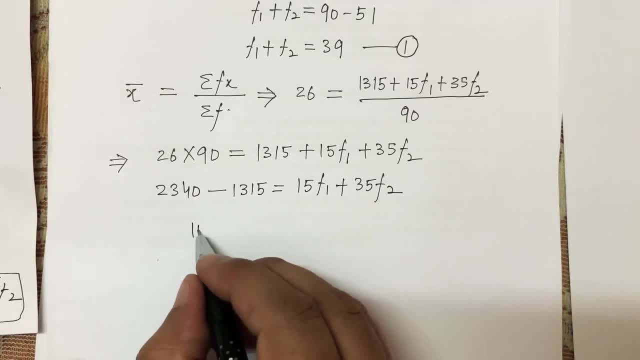 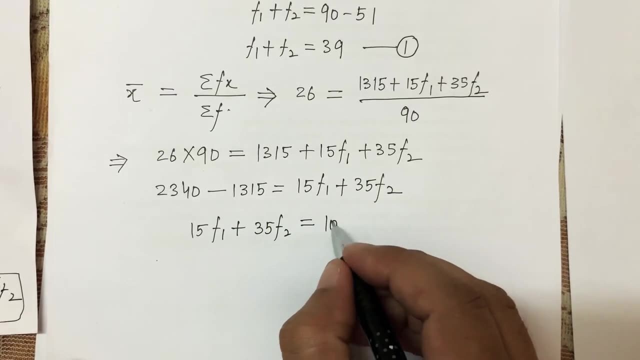 now, if I rearrange the things, it is pretty simply becomes: 15 f1 plus 35 f2 is equal to 1025. 1025 is subtraction of 2340 and 1315, and this is going to be on equation number 2. 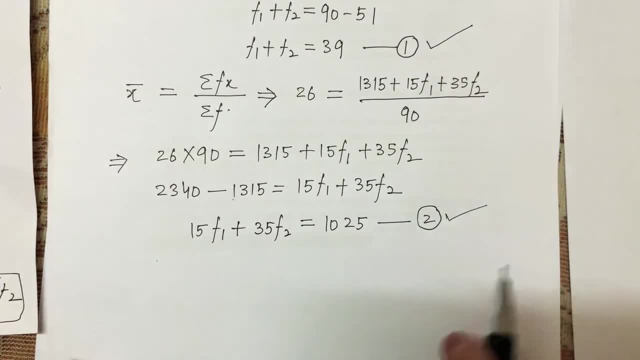 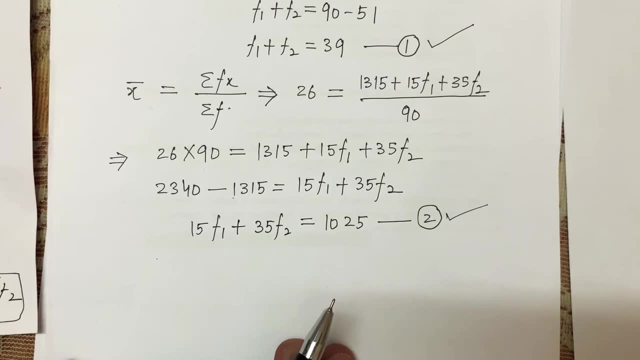 so I'm going to use this equation 1 and this equation 2 to find out the values of f1 and f2. if you could recall the arithmetic you have done in class 8th or 9th, you can easily do that, so I'll just use a fresh sheet. 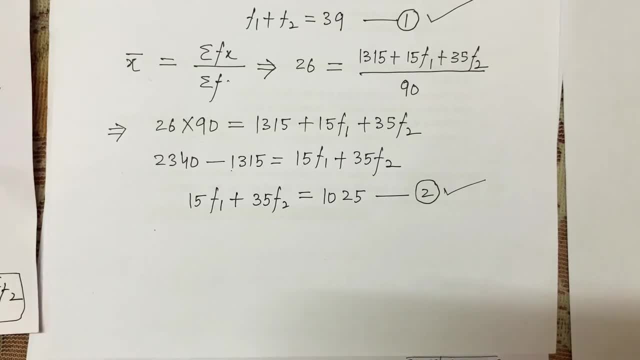 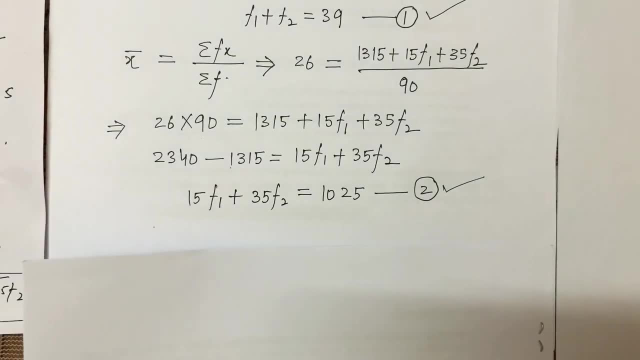 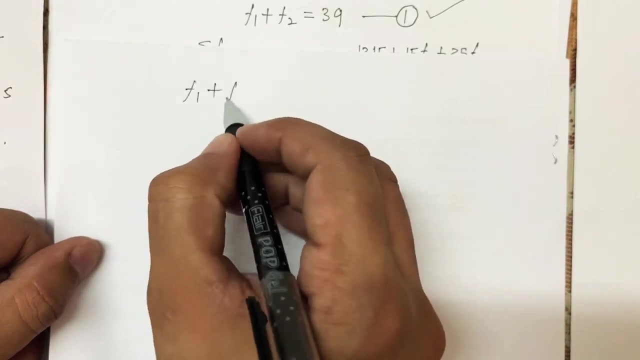 to find out these two particular values, and we just find a white sheet here. yes, I got it, so I'll write both the equations on the sheet once again. my first equation is right here. it is: f1 plus f2 is equal to 39, and the second equation is 15. 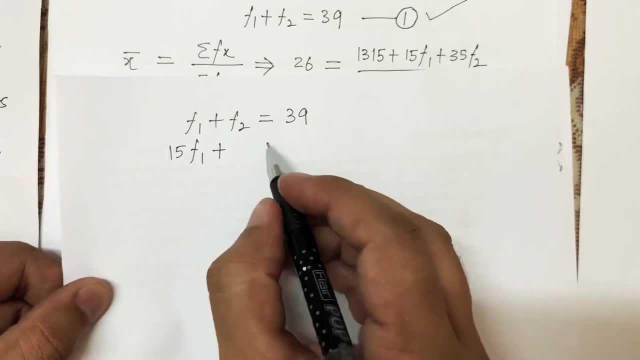 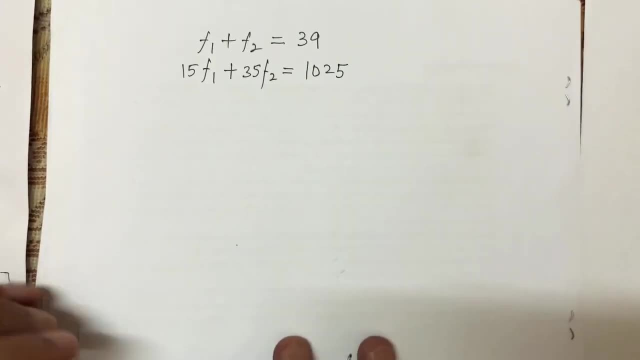 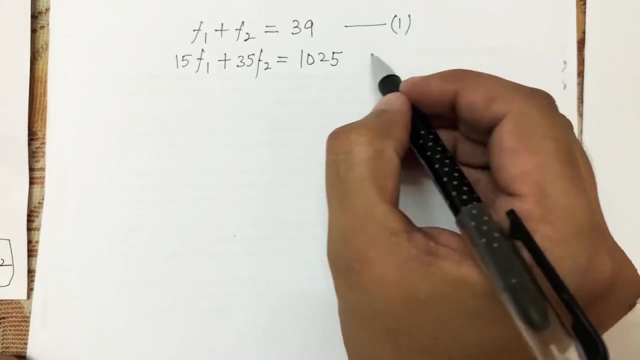 f1 plus 35 f2 is equal to 1025. I'm going to solve them. so what I'm going to do is I'm going to multiply first of all left and right hand side of equation. so I'll just nominate them once again. equation 1 and. 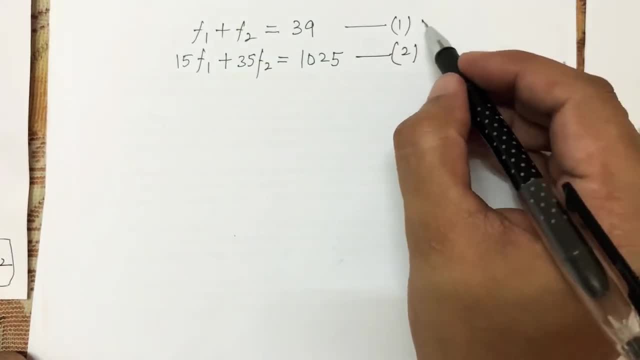 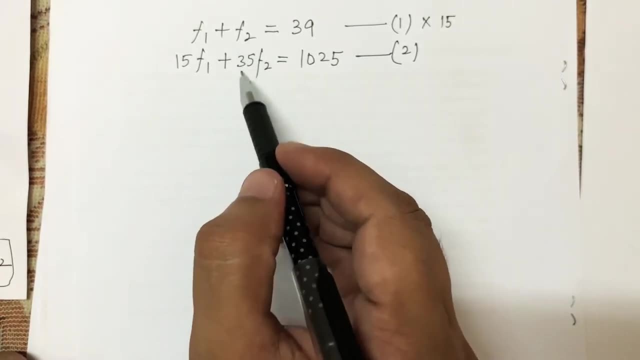 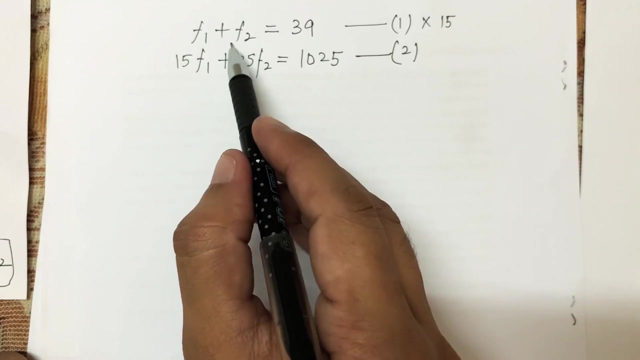 2. so I'll multiply the first equation by 15, both left and right hand side. why do I do that? either I make f1 equal or f2 equal, so I can choose to multiply it by 32. then the f2 multiplier in equation 1 becomes equal to. 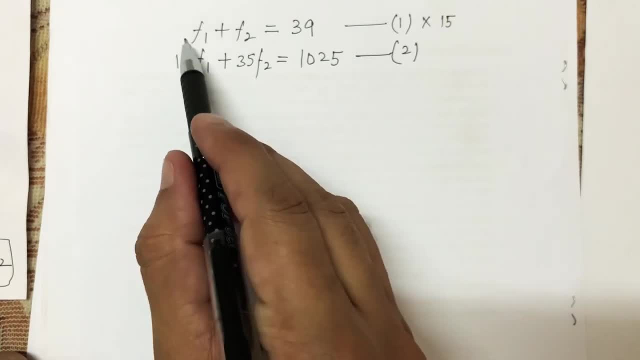 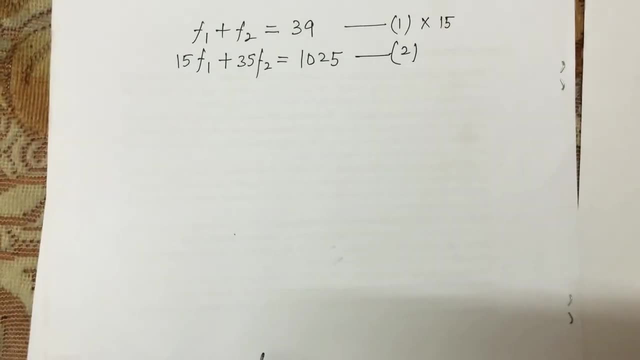 f2 multiplier of equation 2, or I can choose to multiply by 15, since 15 is a smaller number than 35. so for calculation convenience I have taken 15. okay, let's go ahead so if I multiply 15 in equation 1 on both sides. so first equation: 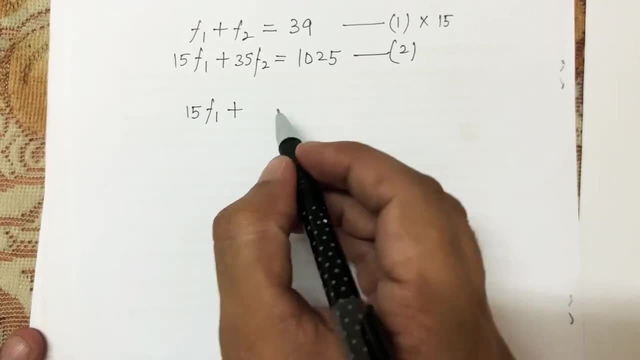 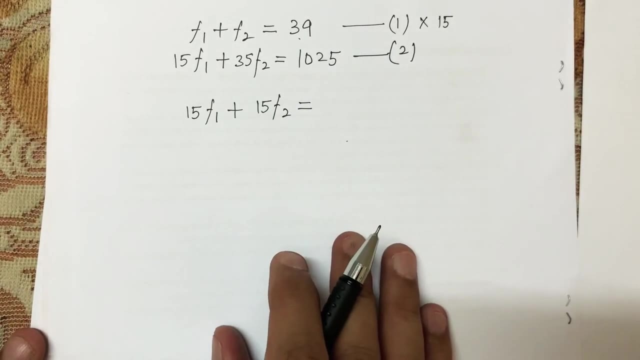 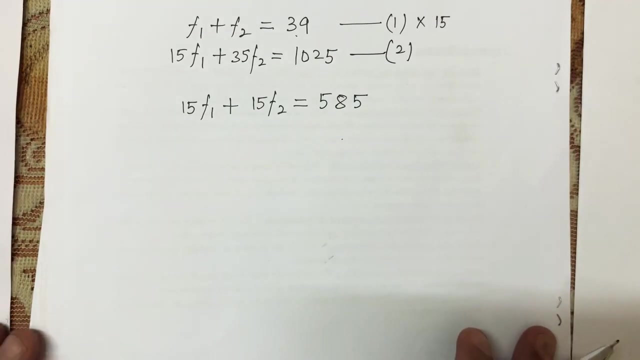 now will become: 15 of f1 plus 15 of f2 is equal to 39 times 15. so what is 39 times 15? it is equals to 185, and this is the greater equal to 611.. so now I can equate it here. 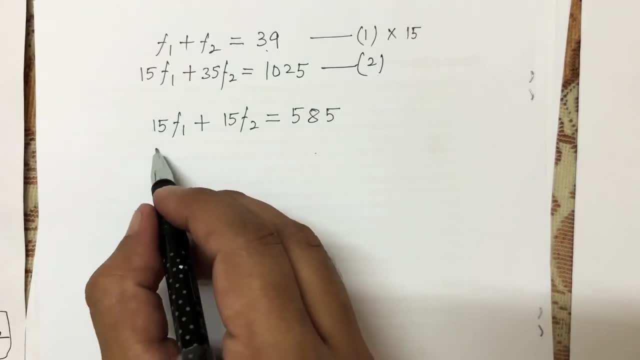 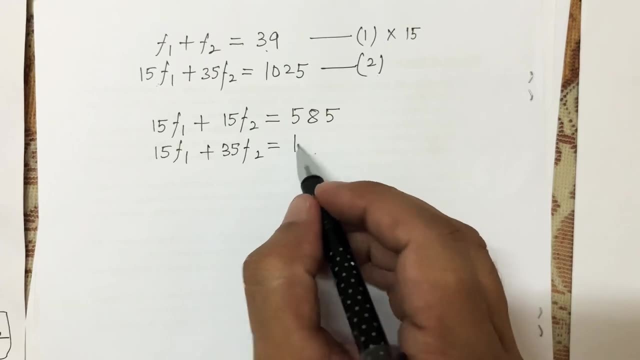 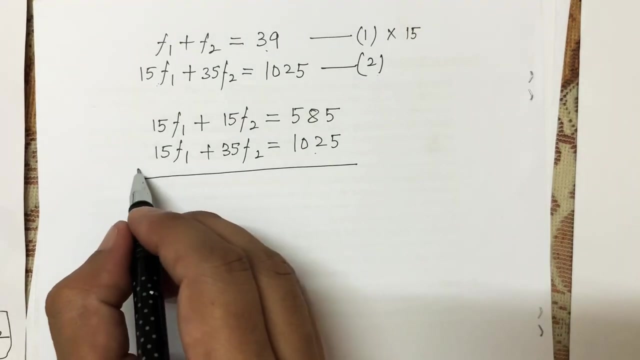 for 15, perhaps one by 15 plus 35 f1. what? because we have already done differing 1025. now what I am going to do is I'm going to subtract and multiply this equation. now you are watching the equation from the outside, then you will notice that it very many times 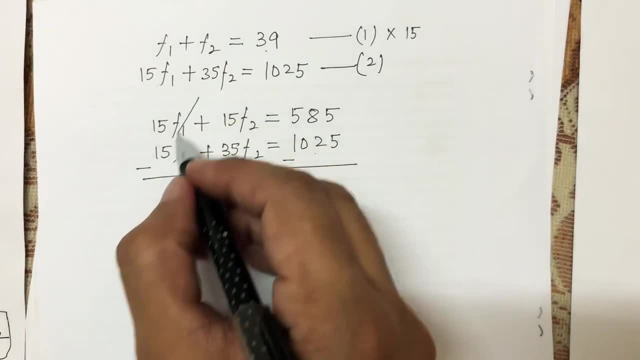 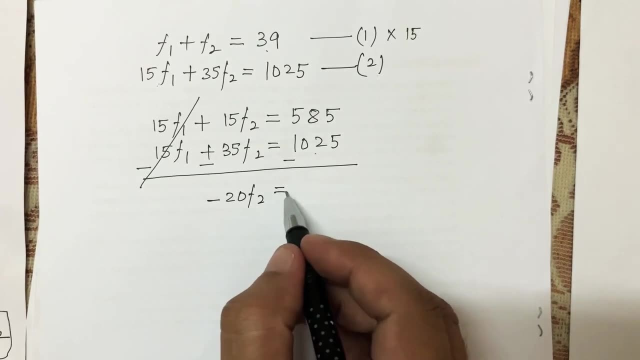 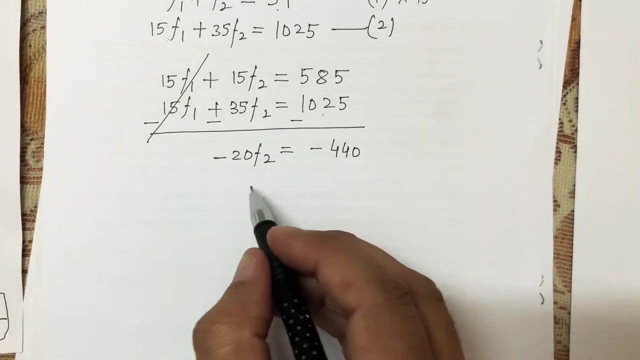 either my first equation or the next equation is 7.2 times 35, less than 251. what does that allow for? minus sign, minus sign. so this is going to cancel out plus minus same. here it is going to be minus 20 of f2 and here it is going to be minus 4, 4, 0. if i subtract both the items, minus minus sign is: 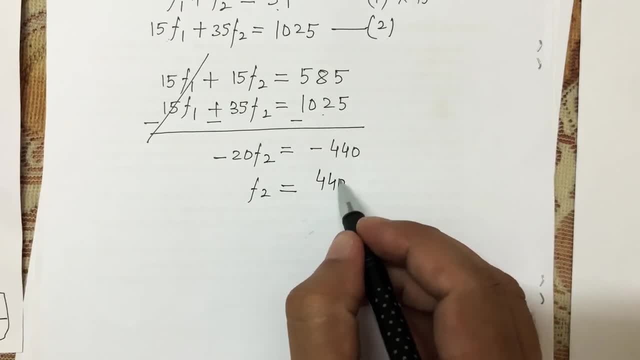 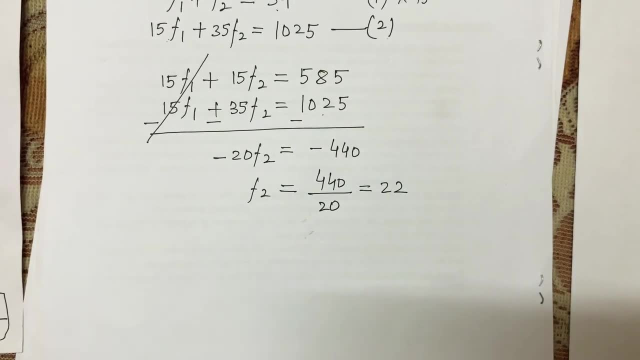 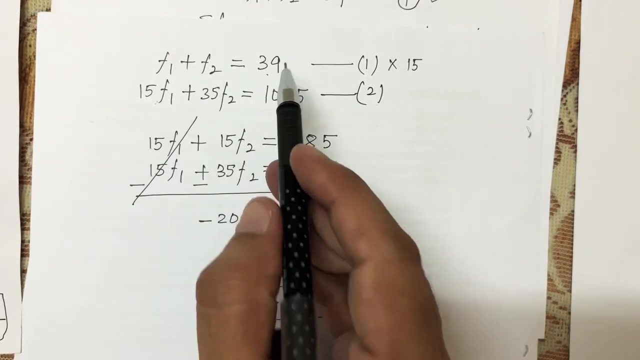 going to cancel out and f2 is going to be 440 divided by 20, which gives me 22. so what do i get? my first frequency. that means f2 value i have got first, which is 22. that is my first input. now i am going to use my first equation right here, where f1 plus f2 is equal to 39. so let's. 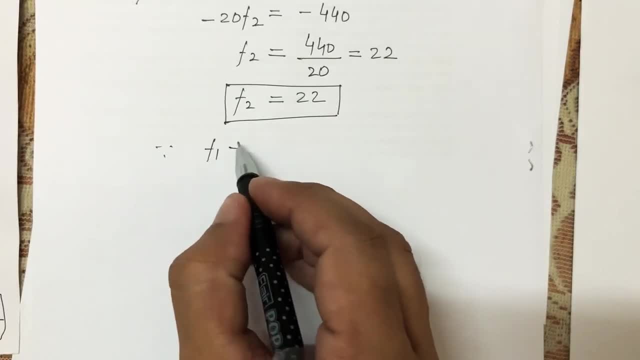 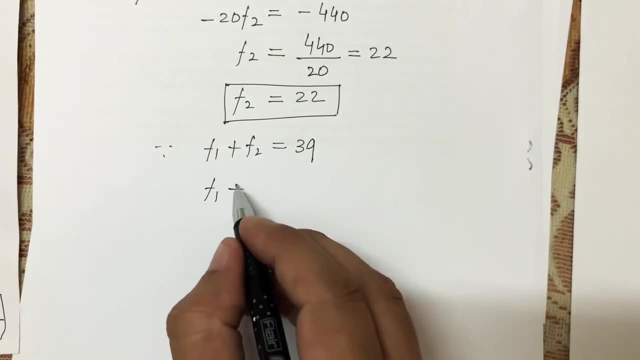 use it this way, because f1 plus f2 is 39. i have already dragged the value of f2, so i am going to supply it here. f1 plus 22 is equal to 39, so i am going to supply it here. f1 plus f2 is equal to 39. 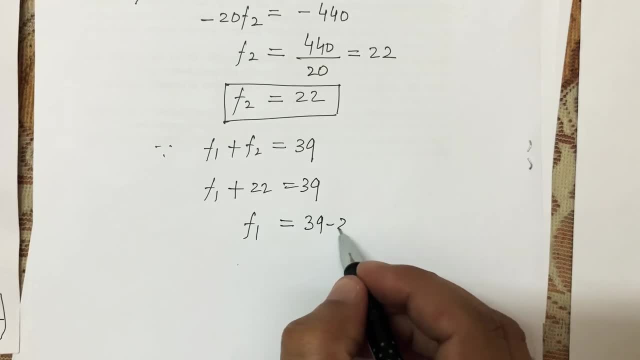 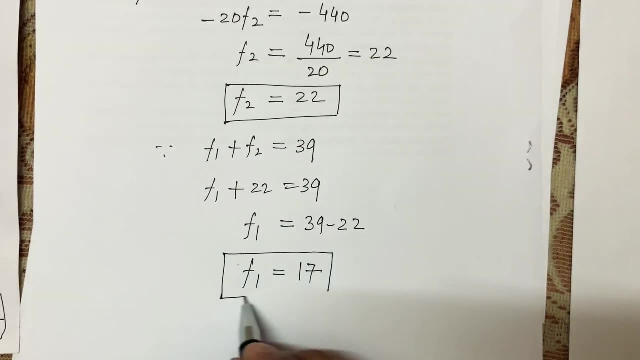 so i am going to supply it here. f1 plus f2 is equal to 39 and f1 but obviously becomes 39 minus 22 and f1 comes out to be 17. so i have my all, both the frequencies, f1 and f2. you can see the calculation once again. you can. 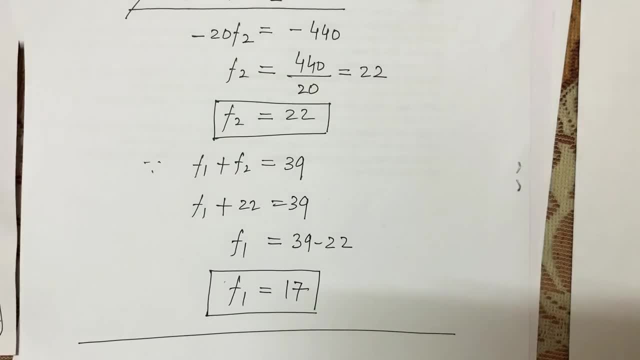 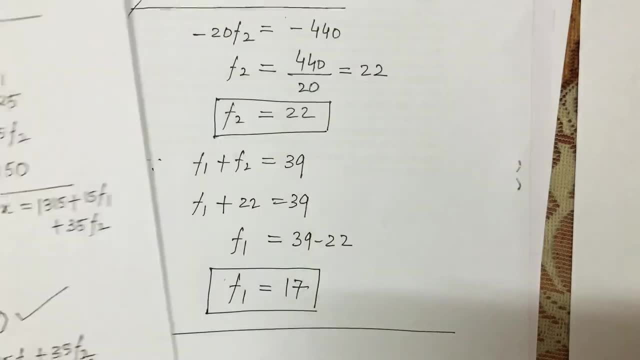 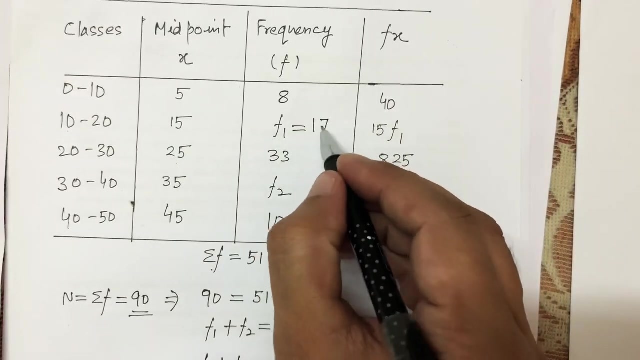 pause the video, rewind it. so i'll fill up these values right here in my original question. so, if you look into this particular question, what do i get as f1? what is f1, 17 and f2 is 22? so i fill it up: f1 is 17, f2 is 22. a little cross check, since i know the total, total number of values. 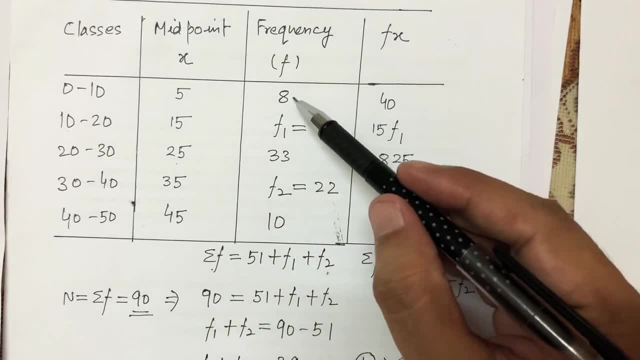 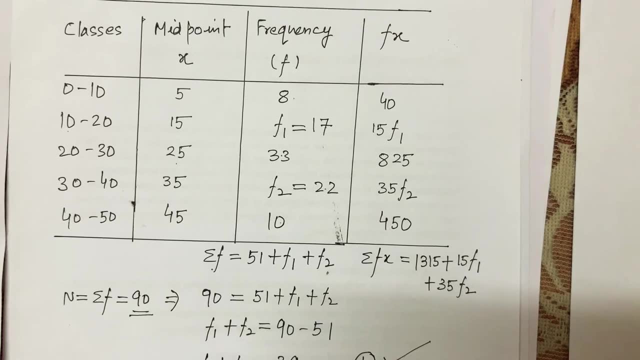 are 90 here, total number of observations. so you can see that 8 plus 17 plus 33 plus 22 plus 10 sums up to 90. so that is it. that's how you can calculate the missing frequencies. thank you very much. i hope the video is helpful for you.